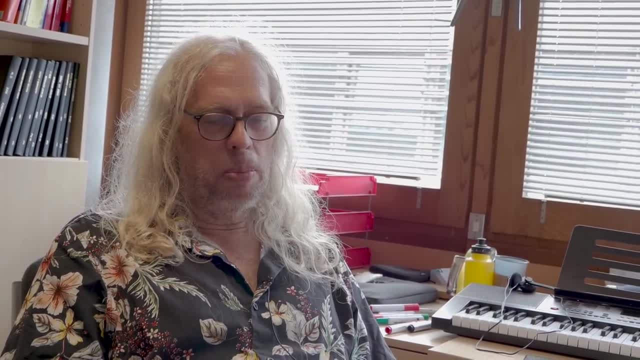 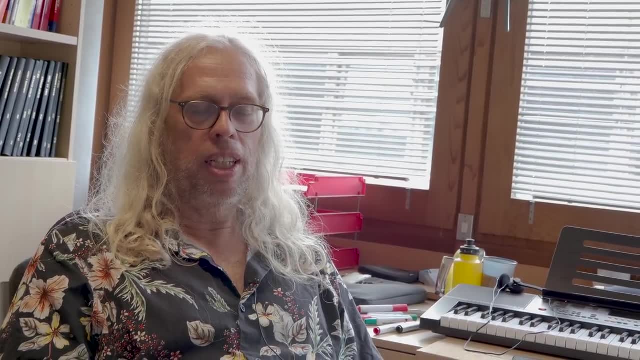 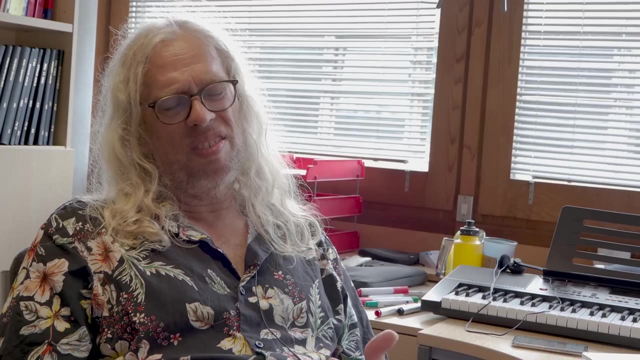 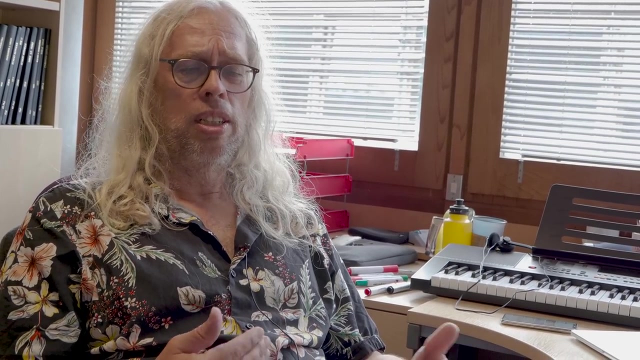 But sometimes we want to be very precise about reasoning and this sort of precise form of reasoning is realized in logic or is investigated, understood and presented in logic. And this is also sometimes quite important to not commit any fallacies, to adopt wrong kinds of reasoning. 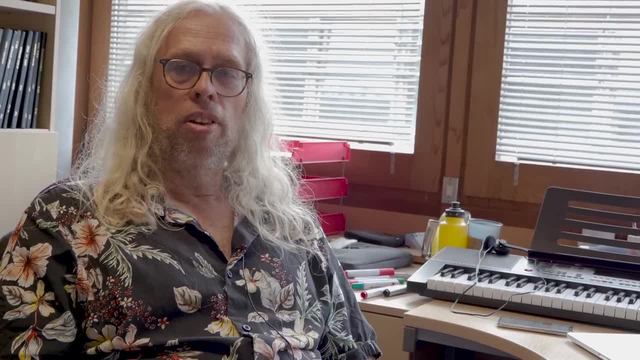 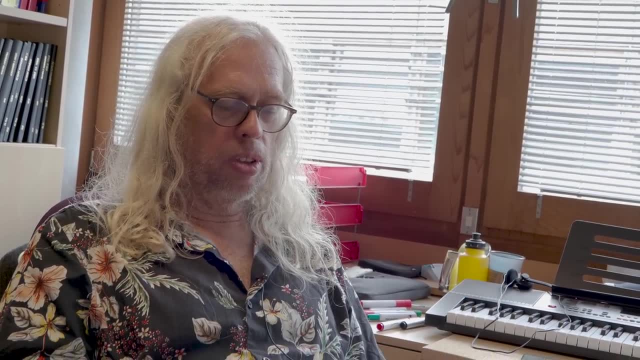 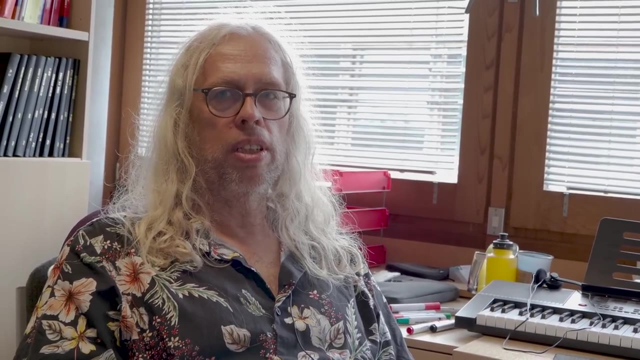 So you really need to understand and study the reasoning, The rules of reasoning. So one of the things I'm doing when I teach logic- so I teach this in the second year- is I'm using a computer program, a proof assistant called Lean. 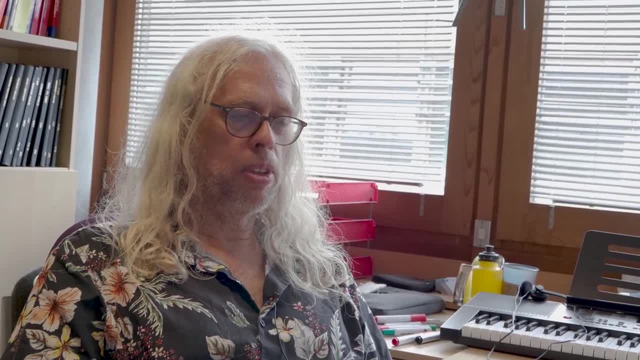 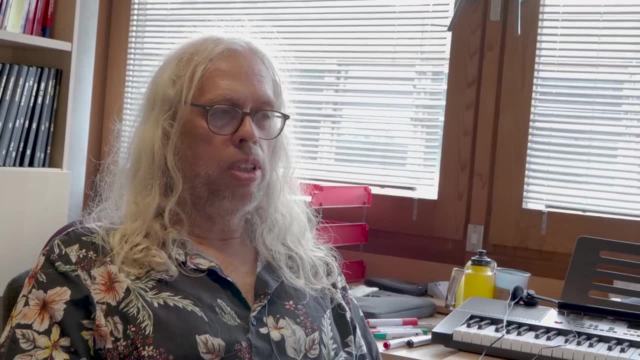 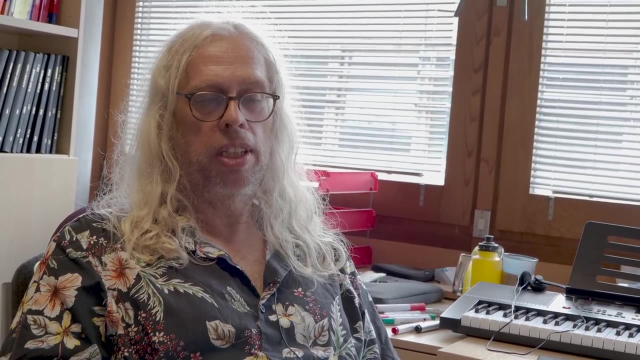 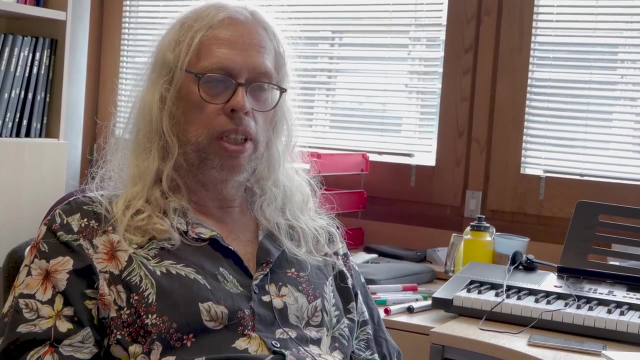 And Lean actually was developed at Microsoft Research by a guy called Leonardo de Mura, who also he developed some automatic proofs and proof systems. He's very famous for the Z3 theorem prover, But then he was also interested in proof assistants or interactive proof systems. 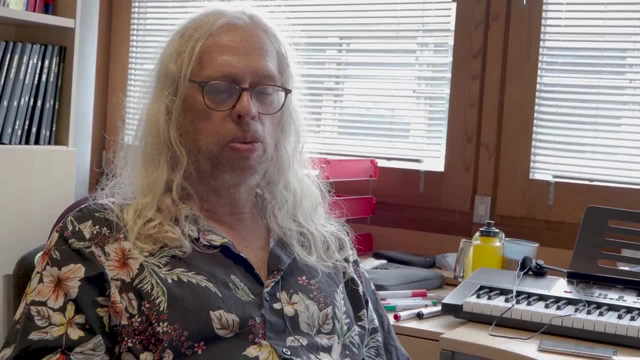 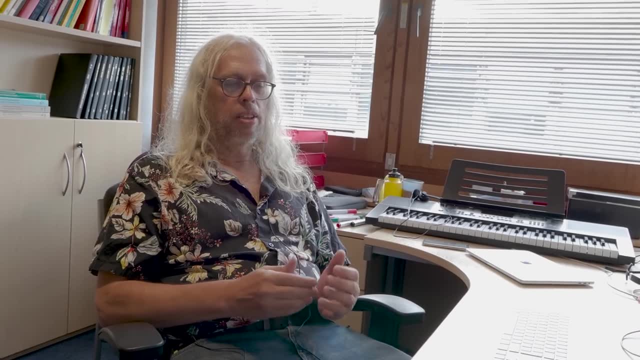 which can interact with automatic theorem proving- And I will explain this a bit more later, I hope, But the main idea here is to have a system you can sort of interact with or an interactive proof system You can type in basically your proofs. 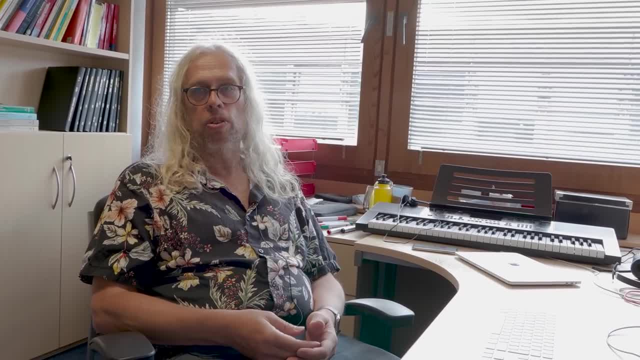 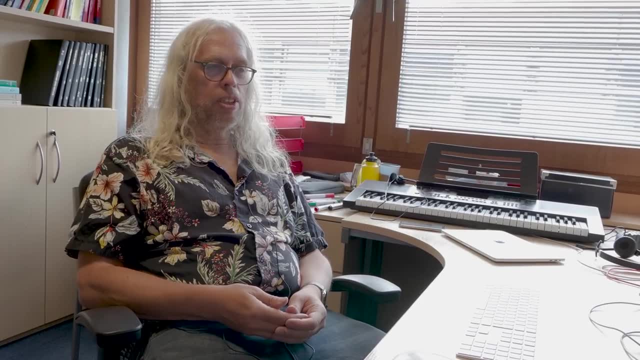 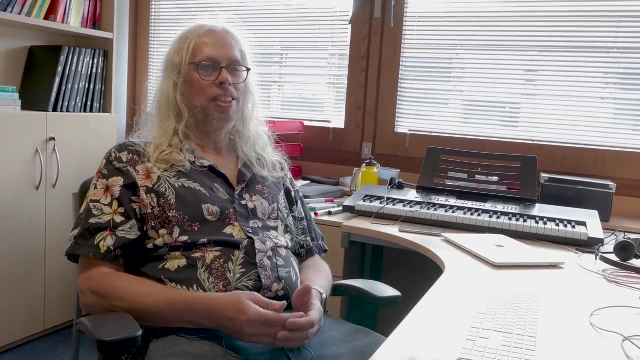 and the proof system will check whether your proof is okay. And when I want to teach logic to students, I find this is extremely helpful, because otherwise it's very hard to say what is really an acceptable argument. I mean people. you give them some examples. 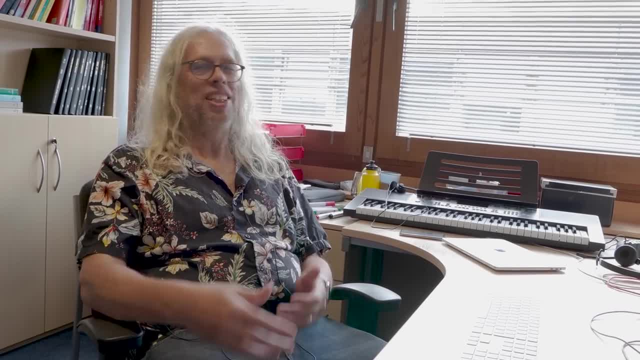 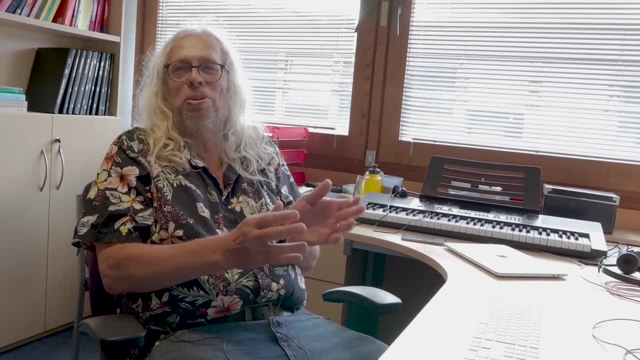 and then you maybe ask for homework, do this, and then they do something which looks like a proof, But you're not sure. you're not sure whether they really understood this or whether they just produced something which they think looks like a proof. 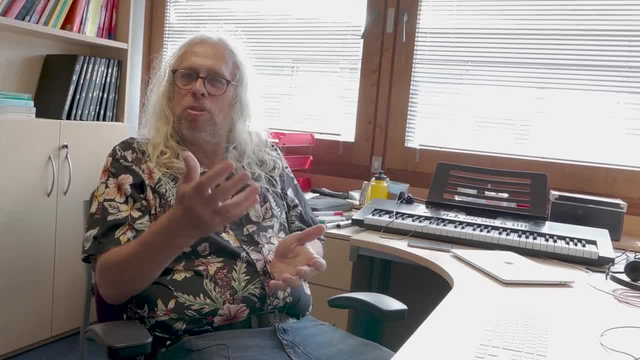 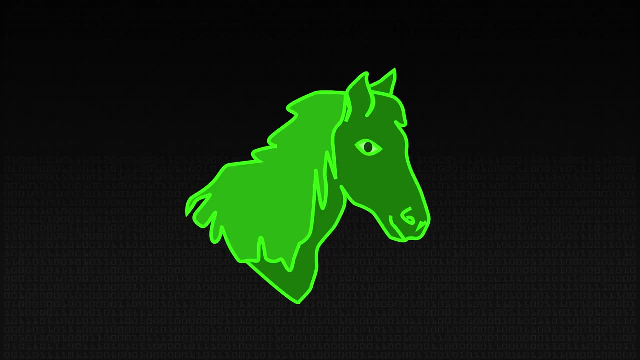 And proofs can be very subtly wrong. I mean, do you know the proof that all horses have the same color? Here's a proof. It uses this idea of induction, So one horse has got the same color right, And now you have any number of horses. 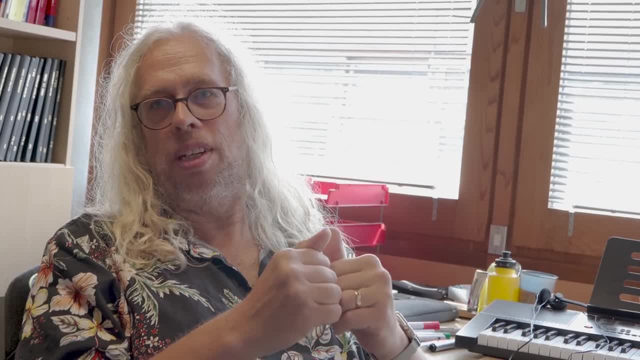 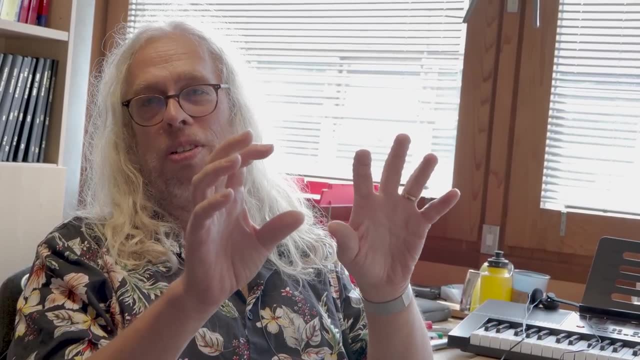 and you divide them into two groups which overlap at one horse. Yeah, And now, by induction hypothesis for the smaller collection of horses, you know that they have all the same color and the horse in the middle has the same color, so the horses together have the same color, right? 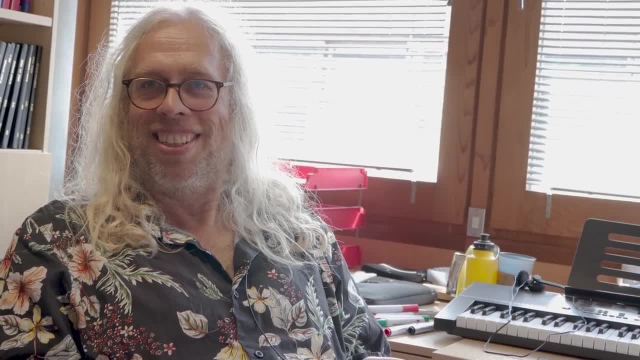 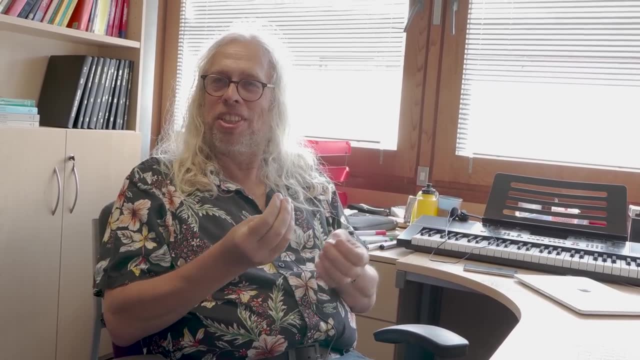 That's a proof that all horses have the same color, right, And this is wrong. Yeah, But these kind of proofs they show up, maybe more subtle. Sometimes you prove something which is actually correct, but your proof is flawed- yeah. 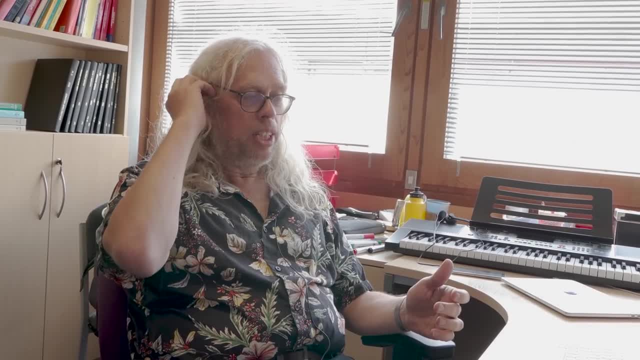 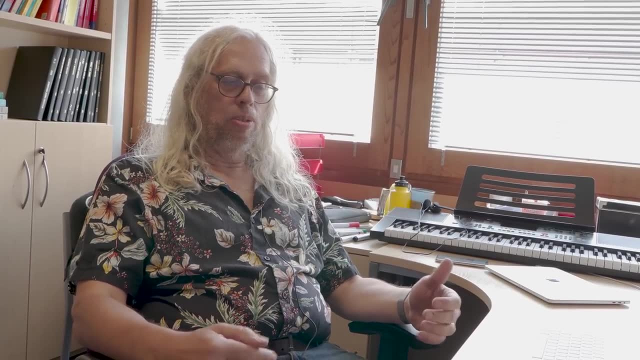 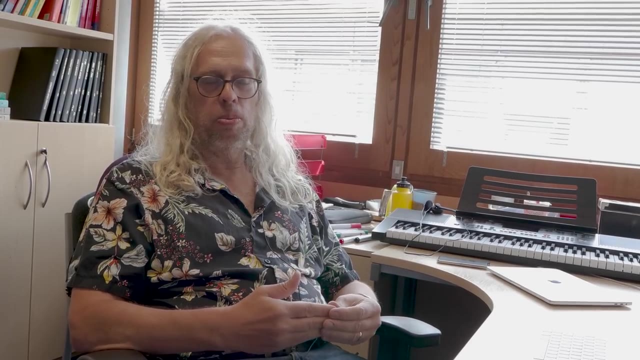 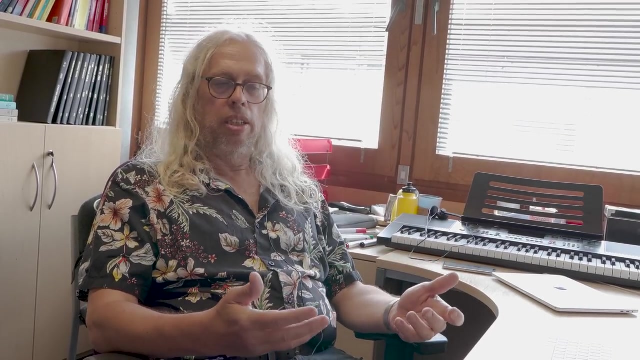 Okay. So I think for me, the best way to explain logic and to make people to understand it is to use these proof systems. Now, they have another purpose as well, because we can use them, and they are actually used, not everywhere, but in some places. 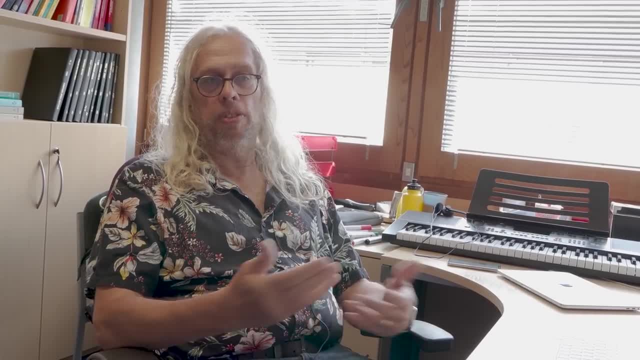 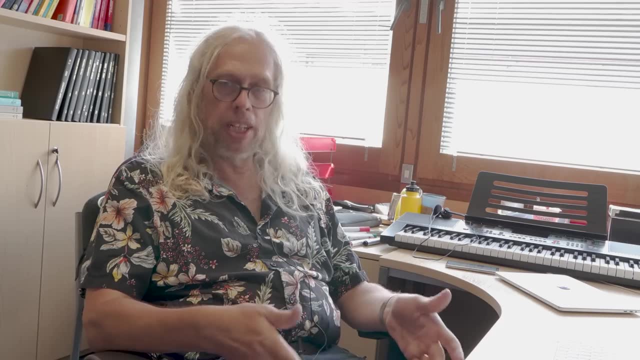 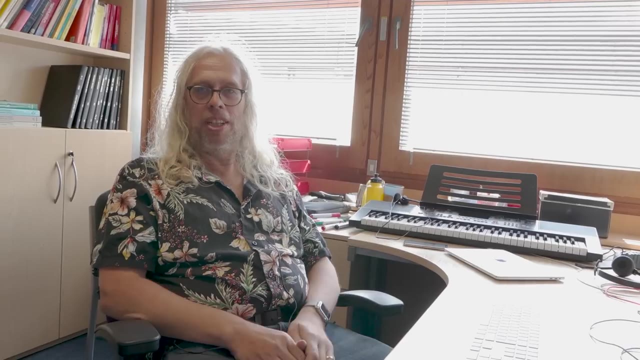 to verify some assumptions which are either sort of safety-critical or which are hardware very frequently used or can be quite failure, can be quite expensive, And so now some companies start to use these proof systems for applications. yeah, The best way to learn it is by doing it. 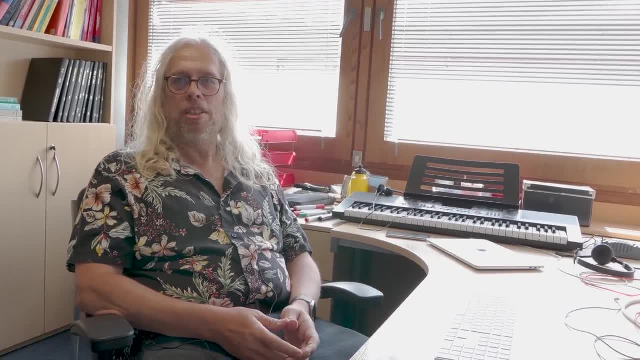 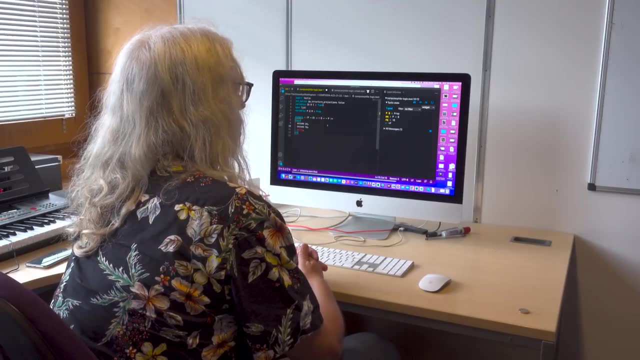 and here sort of a proof system like I'm using is like the lean system which I'm using is extremely useful. Maybe I should say a bit more about lean, which is now also used by the mathematicians. I mean first of all, 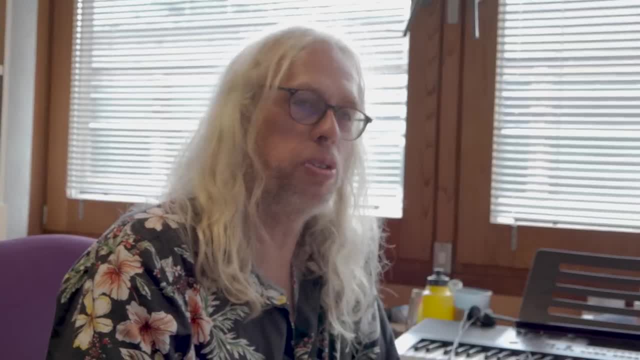 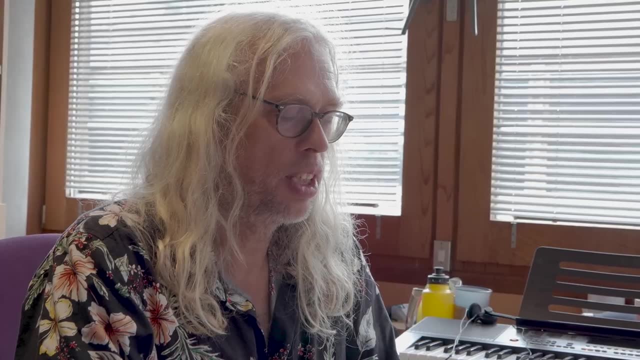 it's mainly used by computer scientists and the mathematicians are a bit conservative. You know they're not. They don't really want to change anything. yeah, But actually there is this guy in Imperial College, Kevin Bothered. 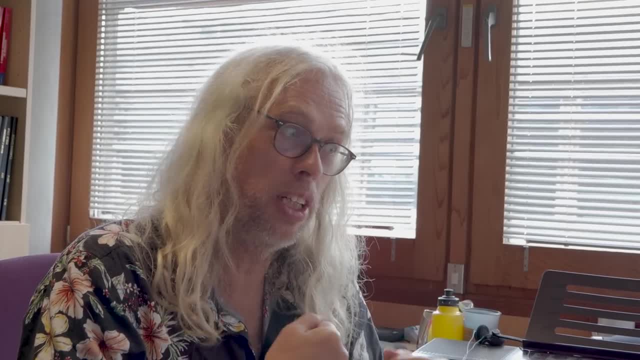 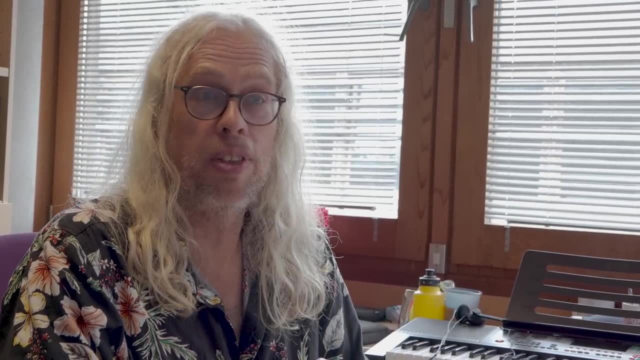 and he is really pushing this and he's using- Although he's using- lean also to teach mathematics to the mathematics undergraduate And he has recently given a talk at the International Mathematical Congress where he has shown what they are doing and it's quite impressive. 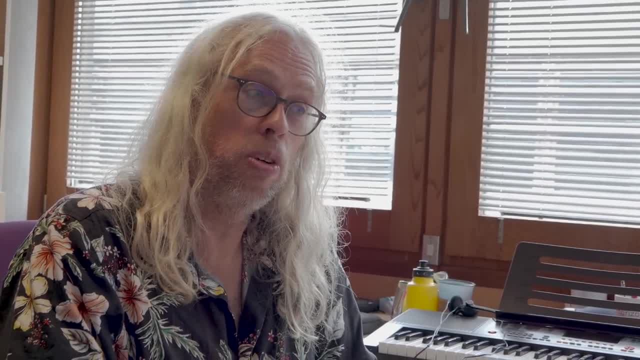 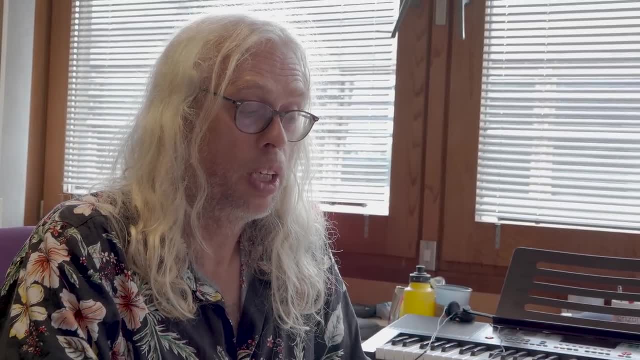 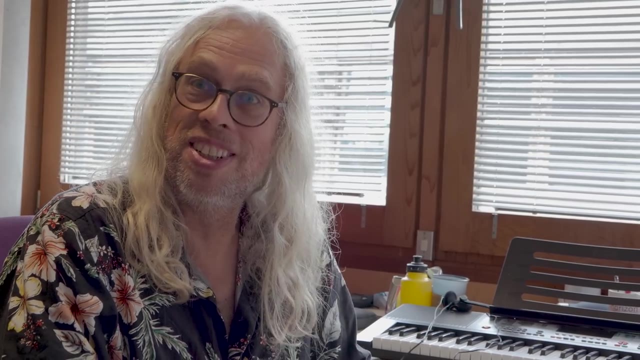 because they're actually able now to formalize very recent results in mathematics using this system and do it with this proof system. And this is impressive because these recent results, they are like icebergs. yeah, There's lots of underwater stuff, lots of theorems that they need. yeah, 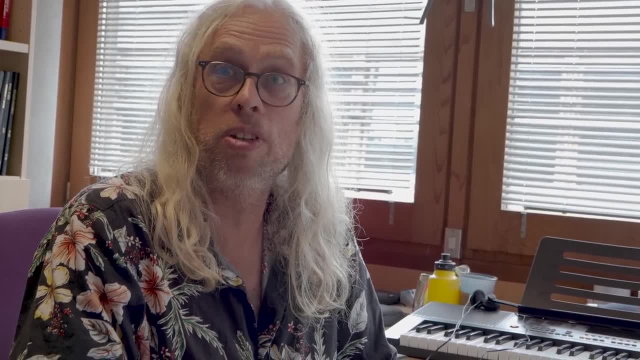 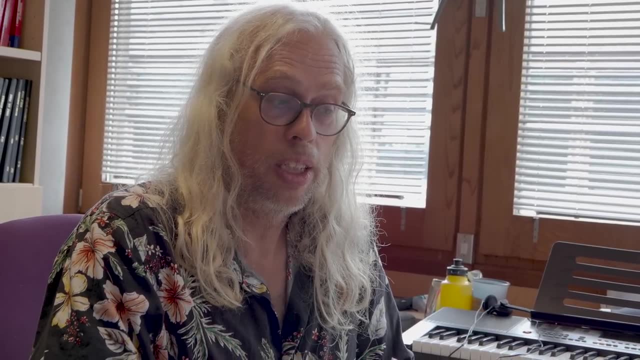 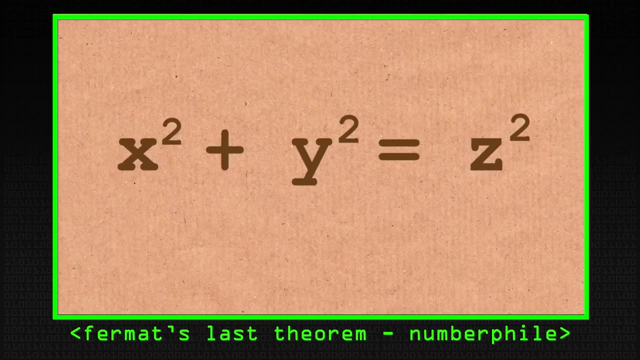 And they have done it all the way down for very recent theorems And really leading-edge mathematics, which is very, very impressive. And now their current project is to formalize, you know, Fermat's last theorem, which says that x to the n plus y to the n. 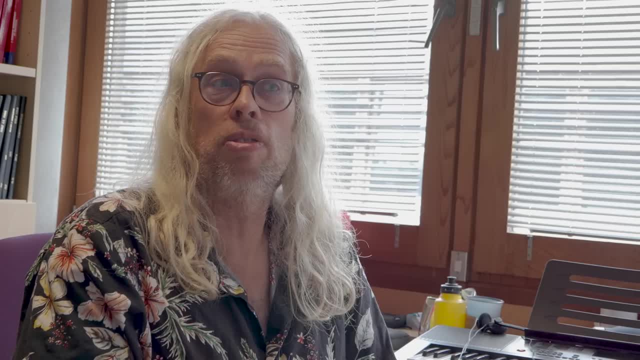 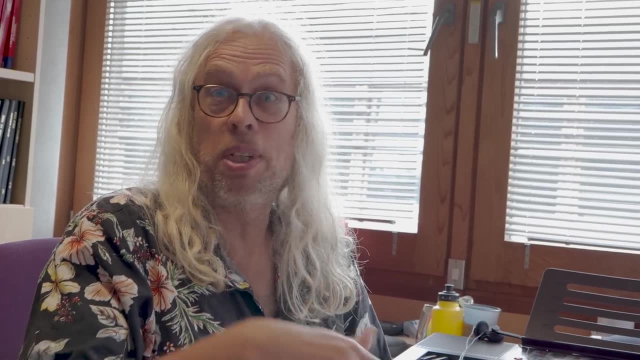 equals z to the n has no solutions if n is greater than 2.. But for 2, we know that 3 squared plus 4 squared equals 5 squared. yeah, But if it's more than squared, if it's cubed or anything higher, 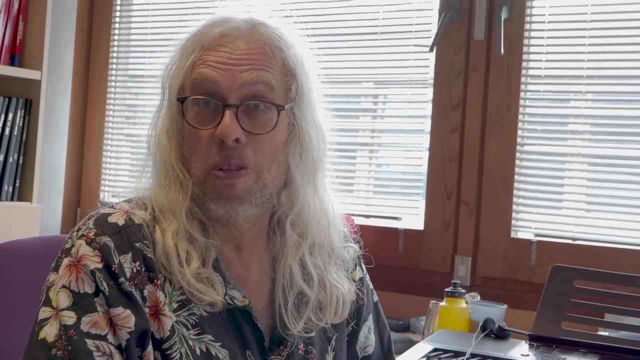 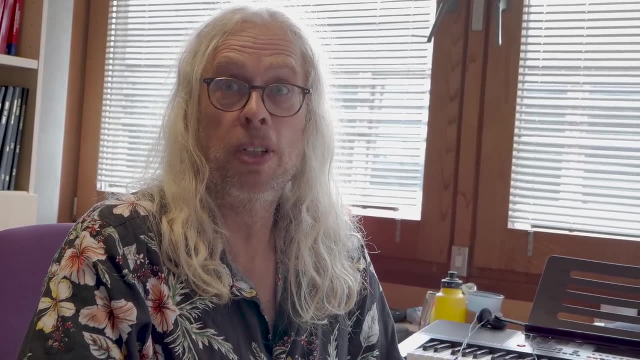 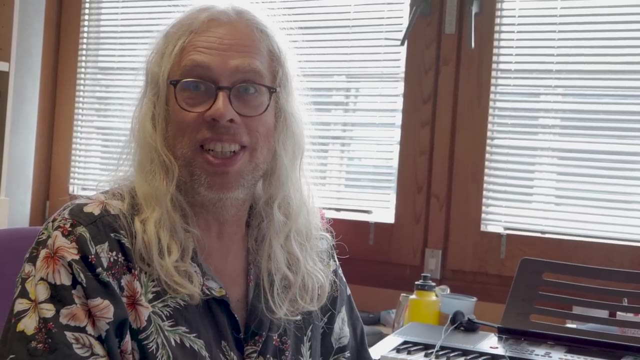 there's no solution, And Fermat claimed that he had a proof. but nobody believes this anymore. But recently, a few years ago, mathematicians came up with a proof, and it's a proof using all of sort of contemporary mathematics. So it's really, really. 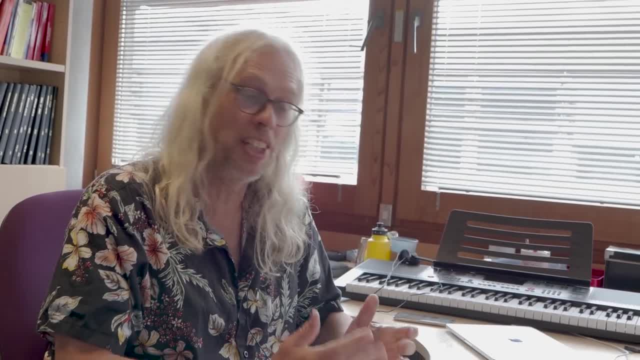 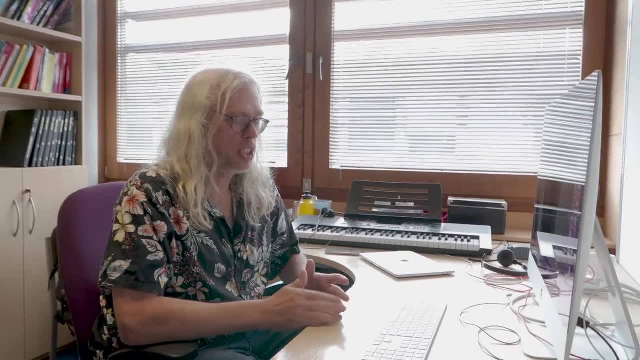 really like a moon landing project to formalize this, and let's see whether they will be able to do this. yeah, Before we do anything very exciting like Fermat's last theorem, which we're not doing today, what we start with is a bit like: 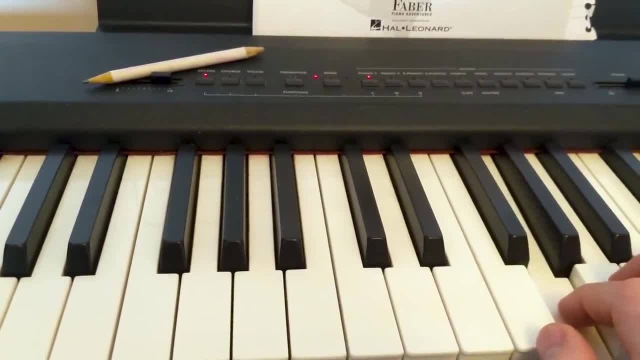 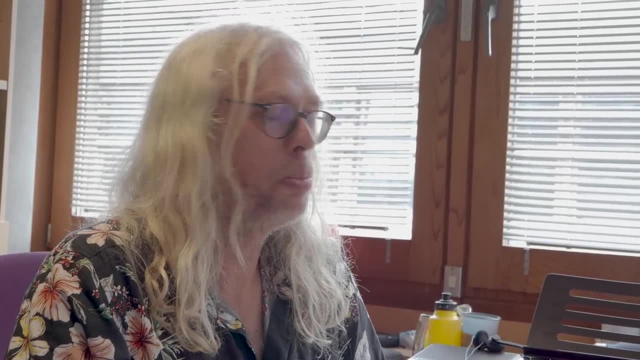 when you do learn piano, you have to play scales right, And scales are a bit boring, but you need to learn them how to move your fingers And in logic we do something like this. We prove propositional tautologies, yeah. 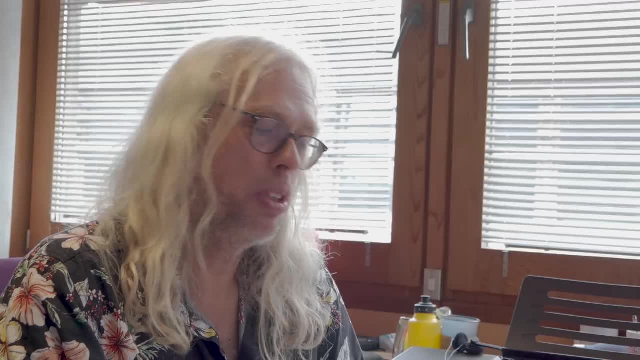 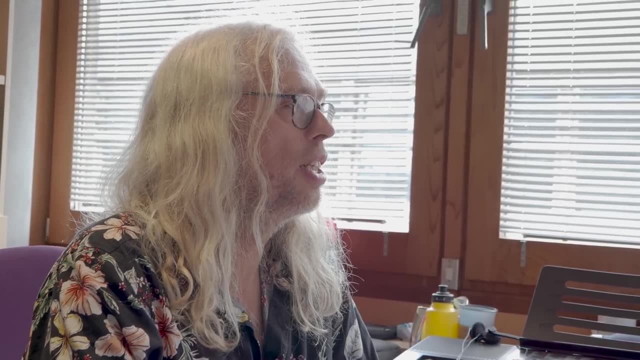 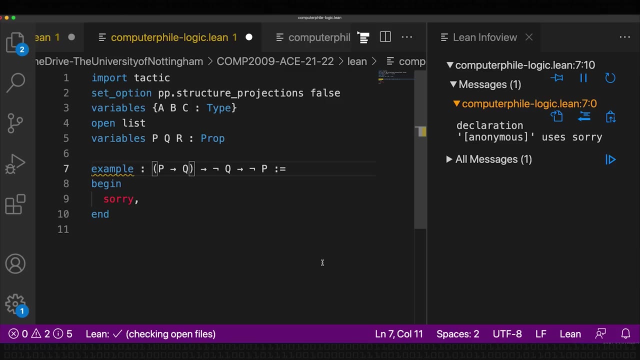 So what's a tautology? I'll give you an example. A tautology is like a propositional expression, which is always true. Let's look at my example here. So I've now launched Lean. Actually, I'm using this Visual Studio Code. 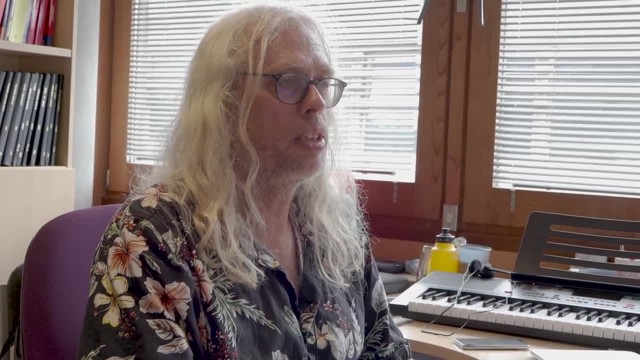 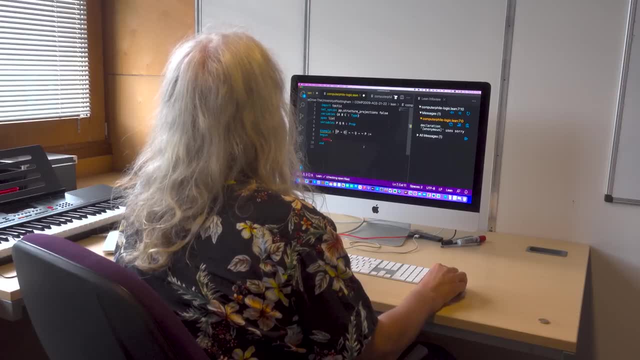 by Microsoft. Oh, I should mention that Lean is free, so you can just download it, And I'm using Lean 3.. There's no new version Lean 4.. Okay, so I've done some stuff there which I'm not going to explain. 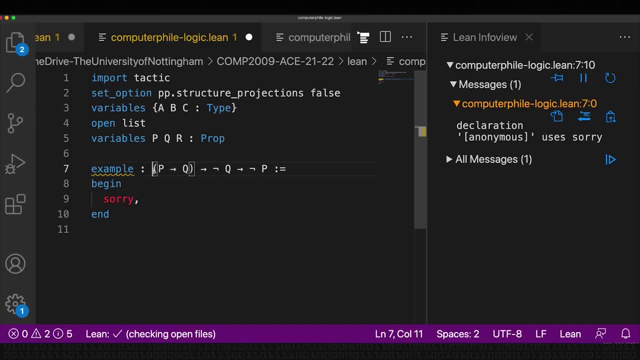 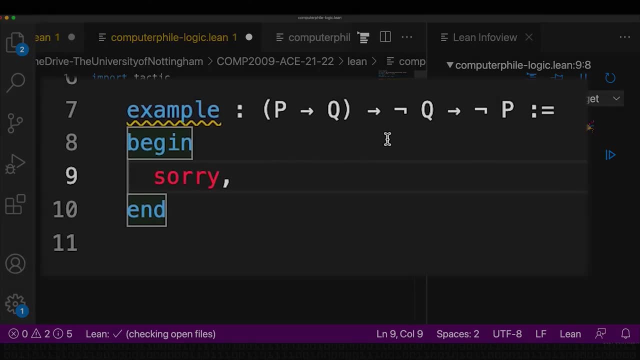 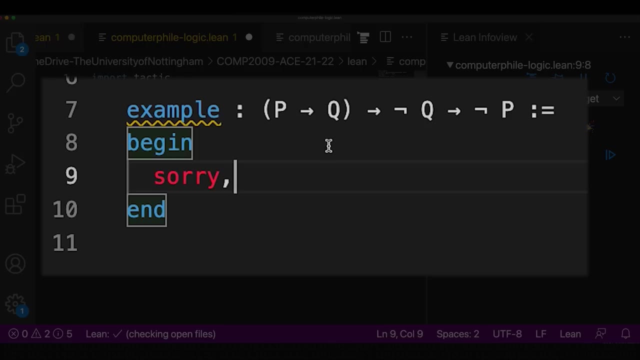 But here is my tautology I want to show. So let me explain this. What does it say? I say here: if p implies q, then not. q implies not p. So this arrow there means implies. so if then, and this little hook means not. 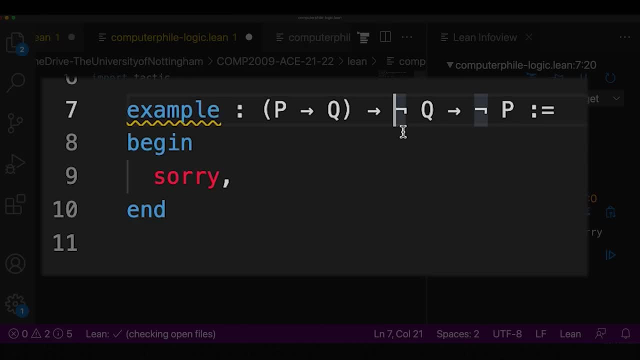 and arrow means implies: And here we could put some extra brackets in to make it more clear, though they're not necessary. So here I'm saying: if p, then q, then, if not q, then not p. So this is a tautology. 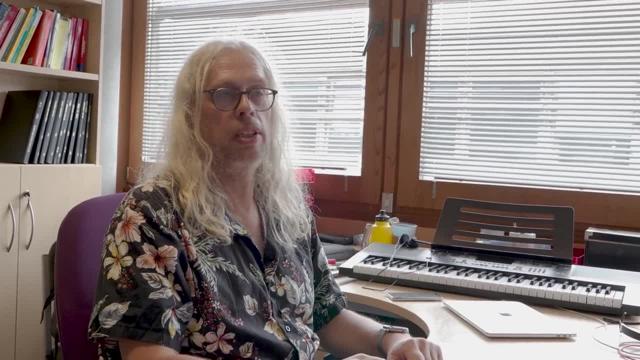 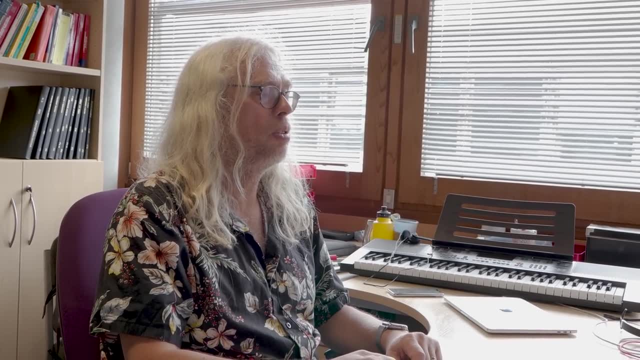 So being a tautology means whatever we plug in for p and q. it's always true, But actually I find when I explain it I find it useful to think of some concrete examples. So let's say p is the sun shines. 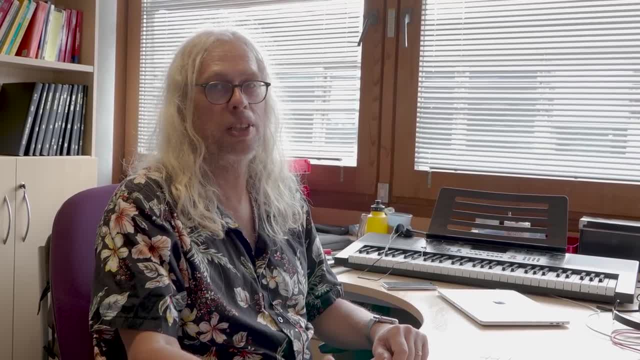 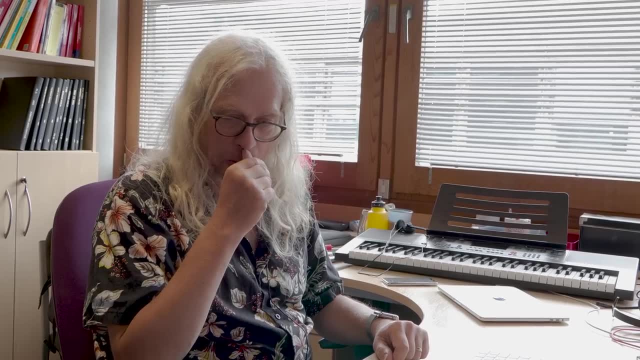 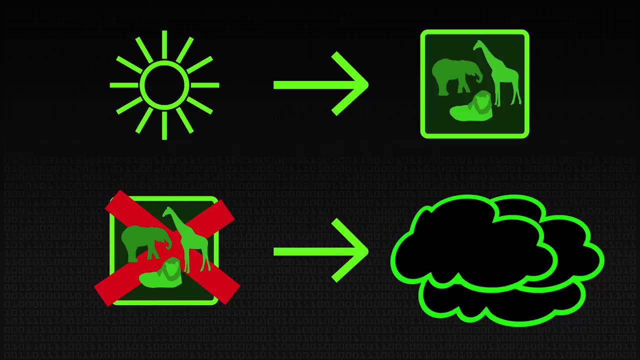 and q, we go to the zoo. And now I tell my children: if the sun shines, then we go to the zoo. The consequence of this is, if we don't go to the zoo, then the sun doesn't shine. And you have to think for a moment about this. 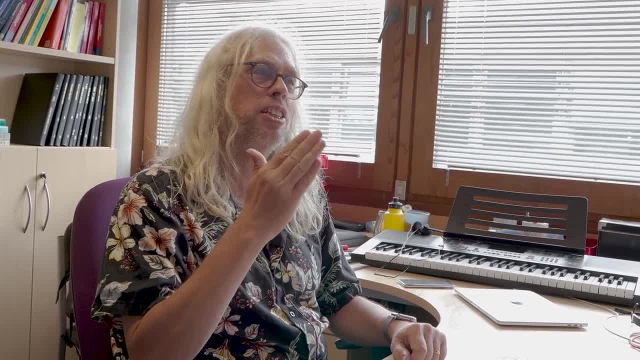 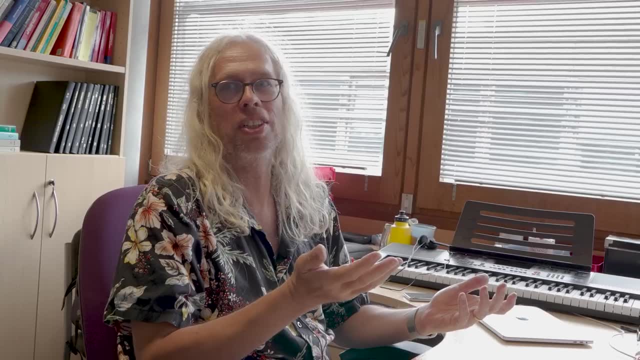 Why is this actually true? If I say, if the sun shines and we go to the zoo and we don't go to the zoo, then obviously the only possible situation is that the sun doesn't shine. For a child, that's probably it, isn't it? 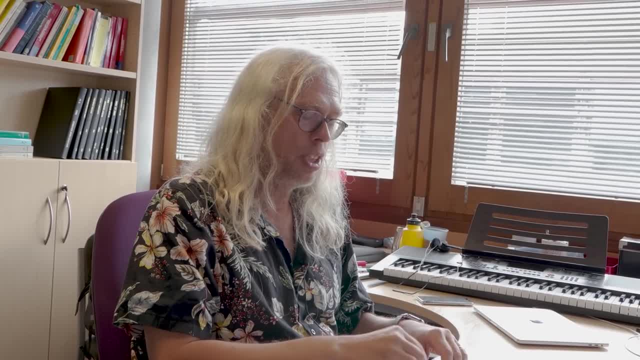 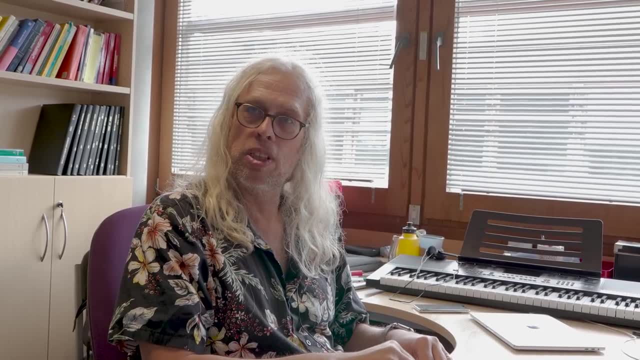 Yeah, not only for a child, I mean. what is not true is: if the sun shines and we go to the zoo does not imply if the sun doesn't shine, we don't go to the zoo because I didn't see anything. 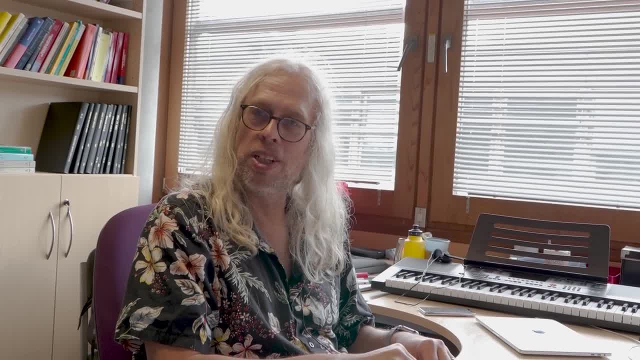 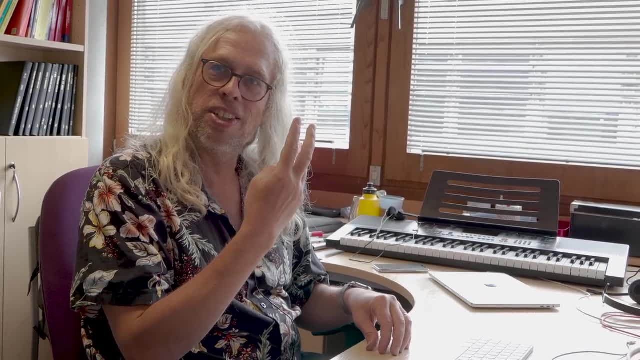 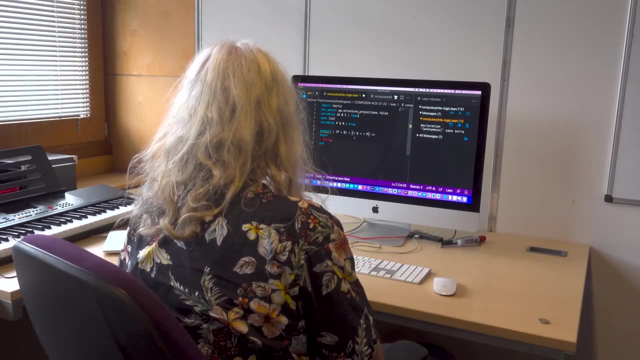 what happens if the sun doesn't shine? That would be a fallacy. But if you turn it around, it's correct. And how can we see? it's a tautology. How can we see it? What do you think? Well, can you factor out those knots? 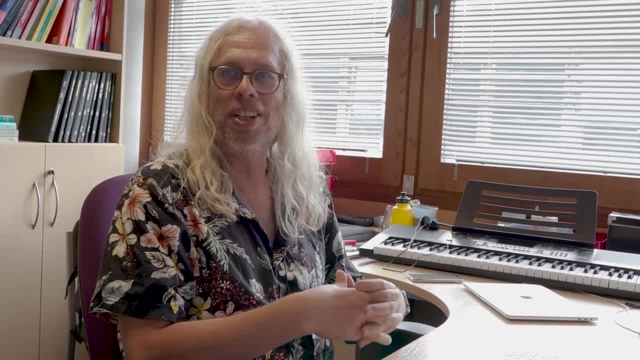 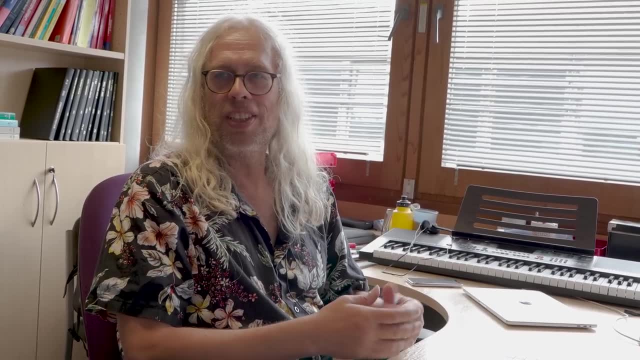 Yeah, you want to have some algebra here. You apply some algebra. Okay, that's one way. It feels like that, Yeah, in general, But people usually have seen truth tables right. Okay, That's another way to check propositional tautologies. 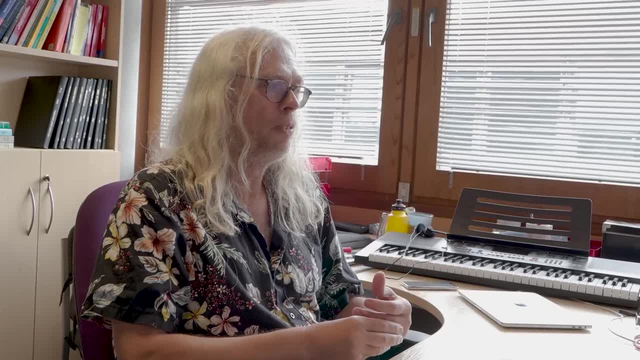 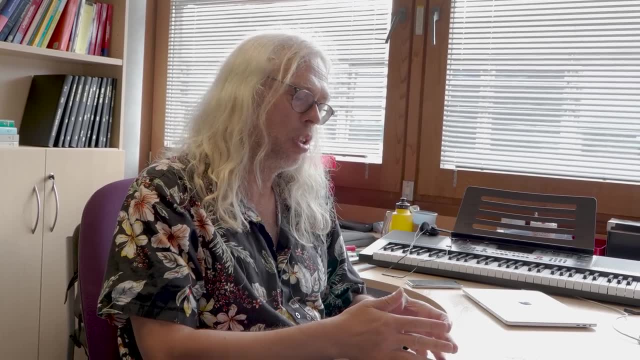 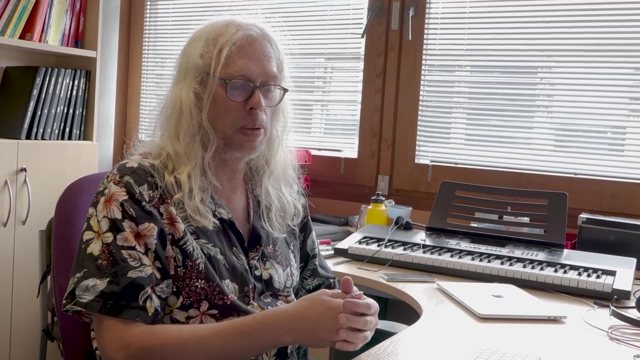 But that's not what I'm going to do today, because actually truth tables are quite okay for propositional logic, But when you move on to predicate logic, when you have quantifiers, when you talk about all the numbers or all lists to do with programs, 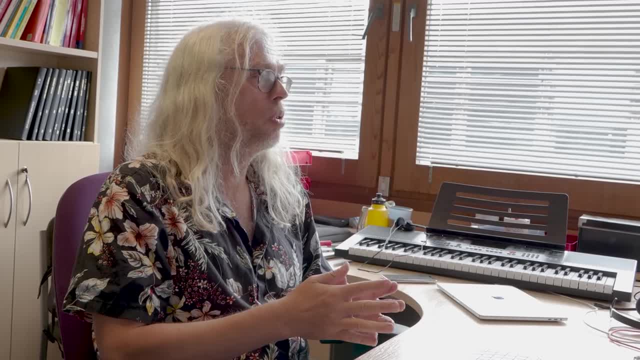 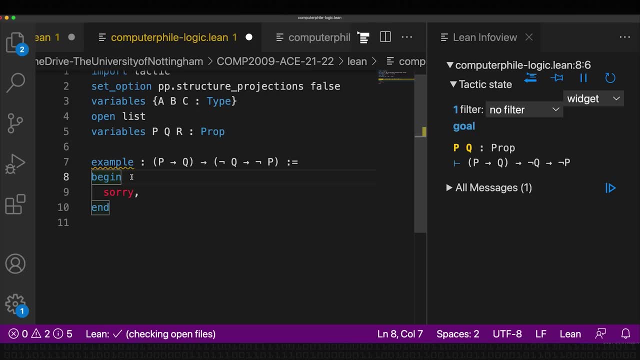 then truth tables are not very helpful. So what we are going to do instead, we're going to look at a proof. Okay, We're going to prove this interactively, And here I said sorry, but sorry means I'm sorry. I haven't yet provided a proof. 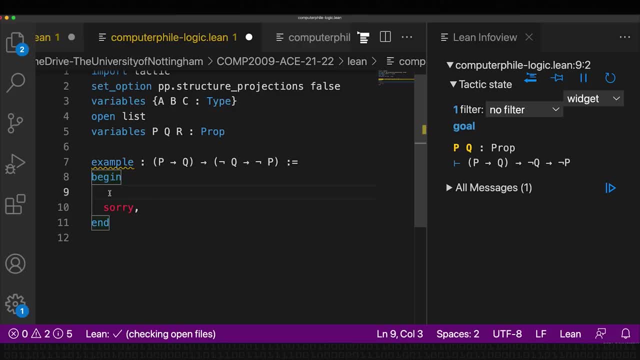 And if I go here into the beginning of this proof block, I'm saying here something. It says: this symbol here is called a turnstile, and that's what I want to prove. This is the statement I want to prove, And it has removed my brackets. 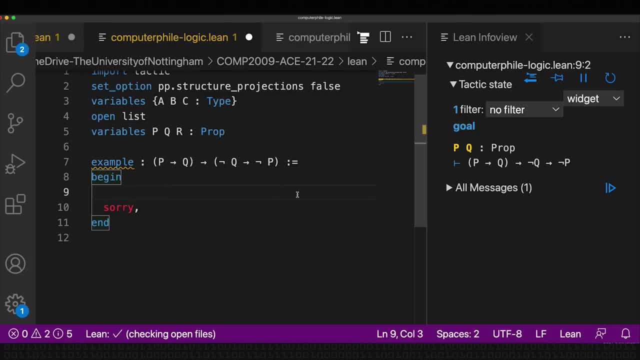 because they're not really necessary. So Lean has done that for you. Yeah, If I go somewhere else, nothing is visible, but if I go here, then it tells me: okay, this is your current proof state. So how do I prove? 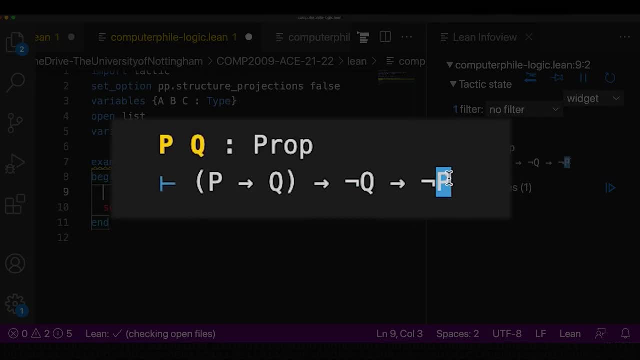 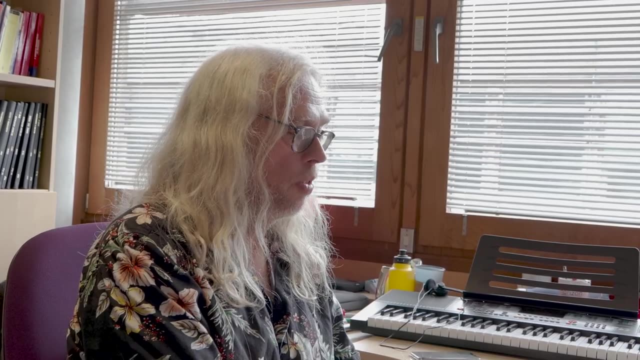 Now I have to prove an implication. So how do I prove? I have to prove. if this is the case, then this is the case. So how do I prove an implication? And the rule how to prove an implication is very simple. I use assume. 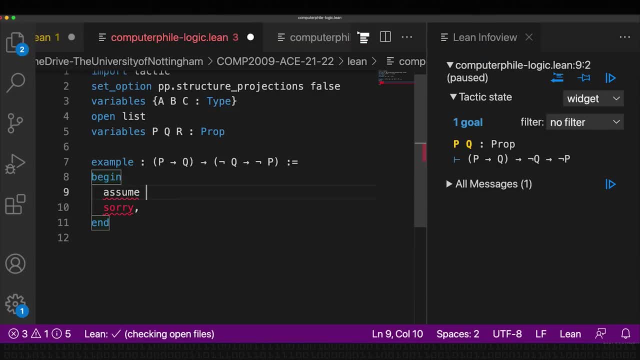 I assume the left-hand side, which I call PQ, and I have to prove the right-hand side. Go on. So what happened now is this proof state has changed. I have to prove only the conclusion. not Q implies, not P, but I have an assumption now. 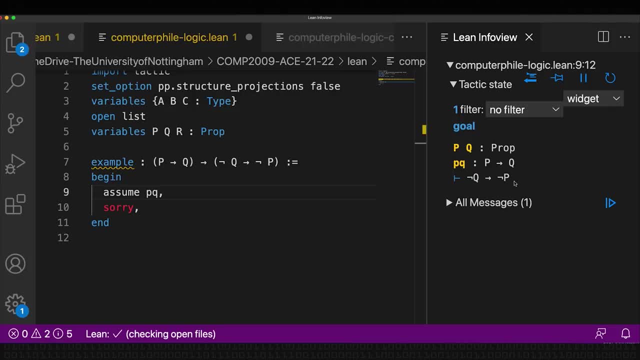 namely that P implies Q. And again I have to prove an implication: not Q implies not P. Now we know already how to prove an implication, namely we assume the left-hand side and we prove the right-hand side. So now, assuming not Q to prove not P. 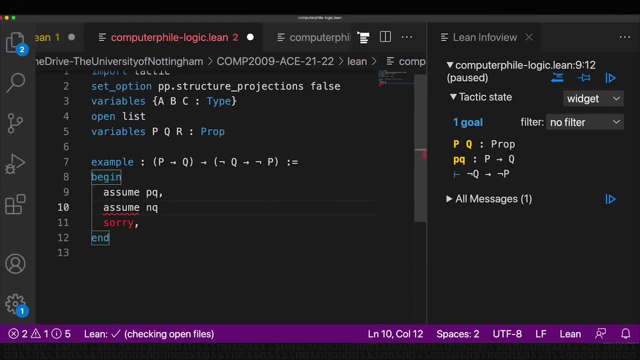 So assume and I call it NQ. And what happens is now that I have another assumption, not Q, and I still have to prove not P. So now we have to understand what negation is. So I have used implication, now we have to use negation. 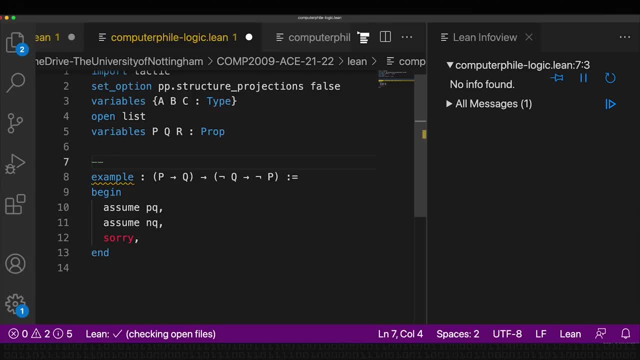 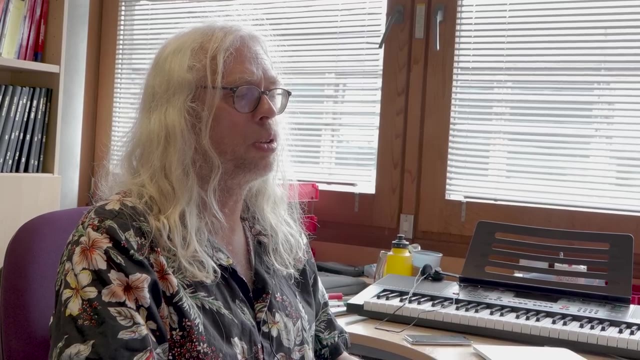 Now let me make a comment here. In Lean, negation is also an implication. It says not P means P implies false. So how can we understand this? False is a bit of a tricky thing to explain, And my explanation for false is: 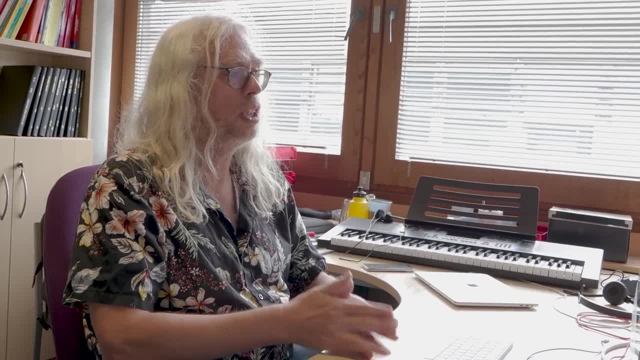 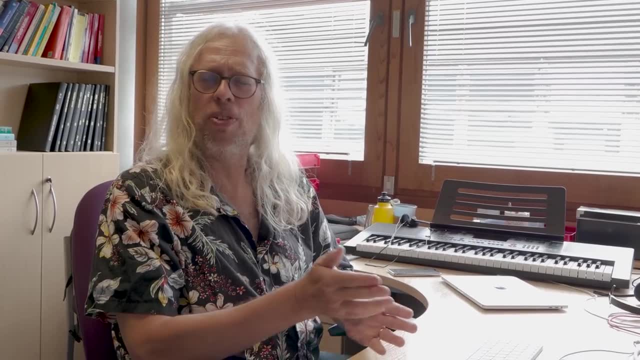 pigs have wings. If I want to say not P, then I say if P, then pigs have wings, And that means not P. If you ask a girl, do you want to marry me? And she says: if I marry you. 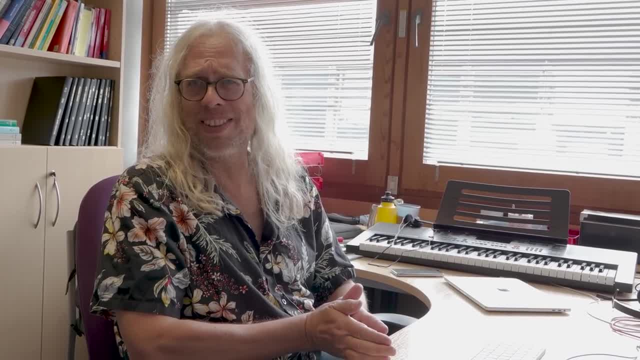 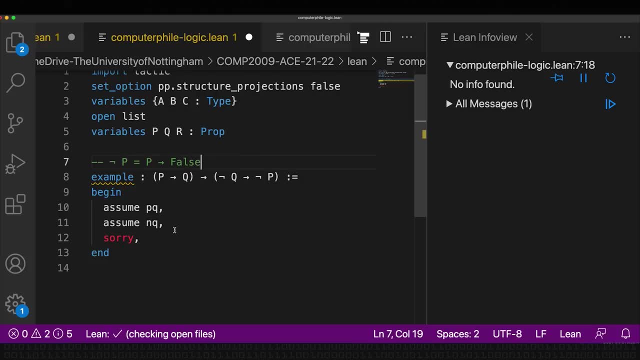 then pigs have wings. That means no right, Yeah, Yeah, Pigs might fly. Yeah, It's not really Okay. So that's the idea, So it's just an implication. So now, in this situation, we are here. 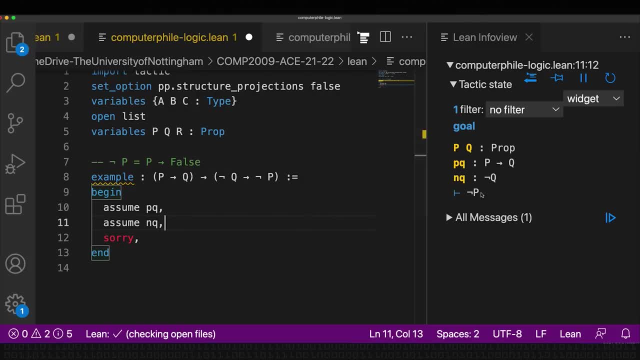 We want to prove, not P, But that really means P implies false. So all we have to do we have to assume P and then we have to try to prove that pigs have wings, right, Okay, So you see, I have to prove the assumption P. 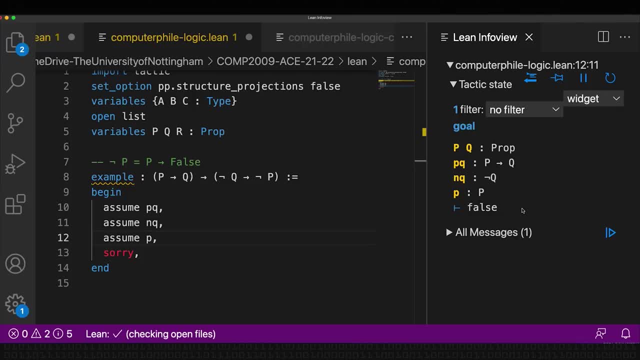 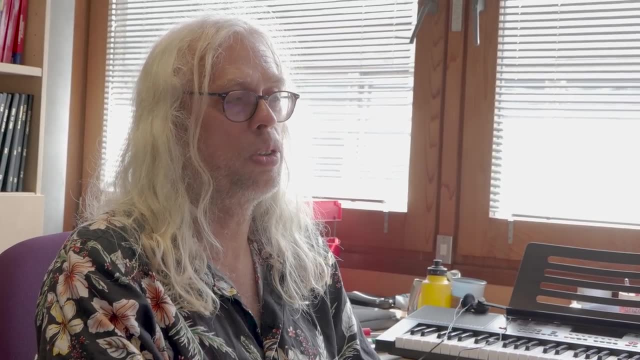 and I have to prove false. So how can I prove false? How can I prove that pigs have wings? Now, actually there's one way, because I have an assumption called not Q, And not Q means if Q, then pigs have wings, right? 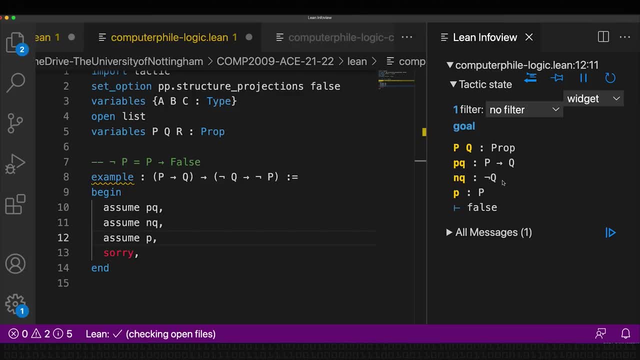 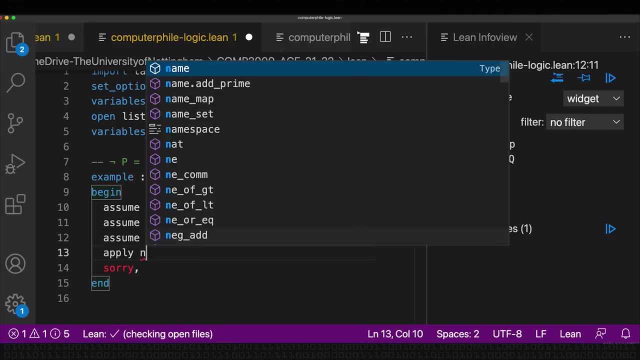 So I want to prove: pigs have wings. and I have already an assumption which says: if Q, then pigs have wings. So now I'm using this. So this time I'm using a different tactic. I'm using apply and apply and Q, And what's happening? 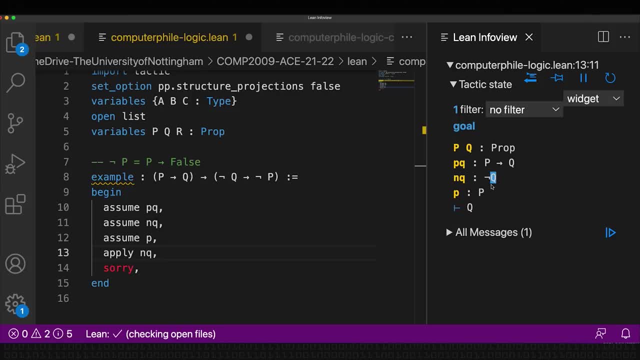 is now I have to prove Q because I wanted to prove if Q. I mean I used if Q, then pigs have wings. Now I've used this. Now I'm down to proving Q. And again, how can I prove Q? 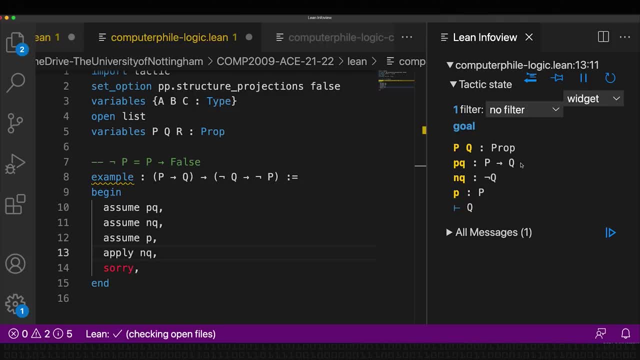 I look at my assumption. There's one assumption which says: if P, then Q. I can use this and reduce proving Q to proving P. Okay, let me just do this. So I say: apply P, Q. And now what happens is: 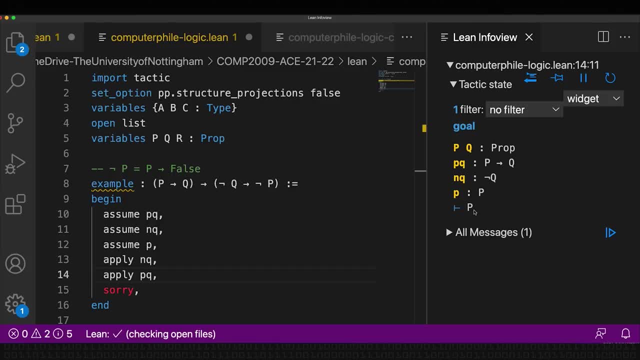 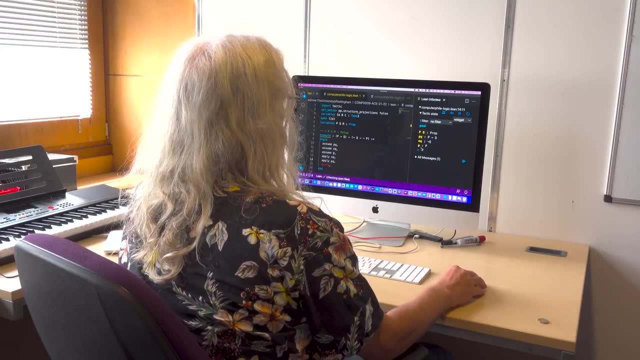 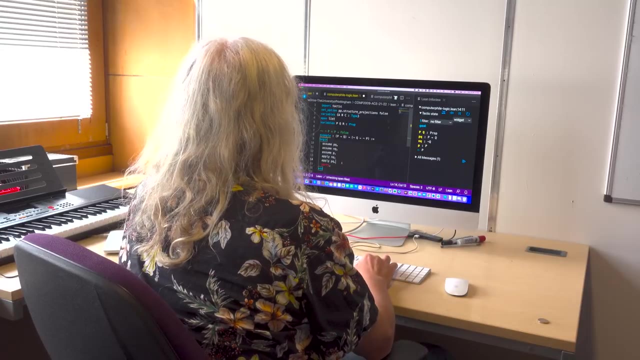 I have to prove P, because if P, then Q. I want to prove Q. Now I'm down to proving just P. But that's very easy because I already know P, I have an assumption P And I can just say exact P. 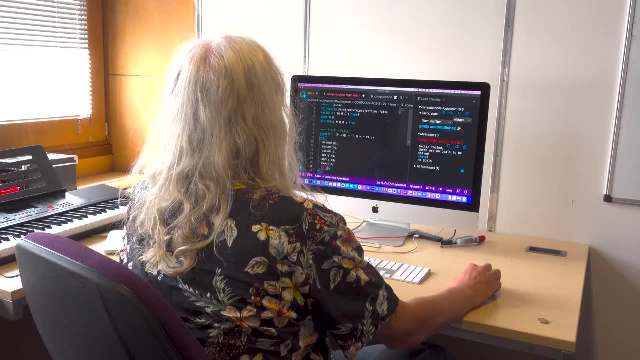 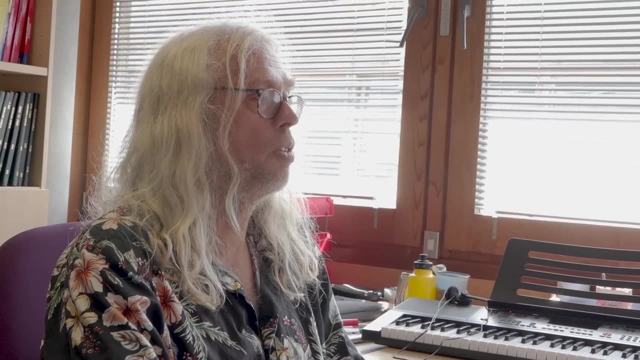 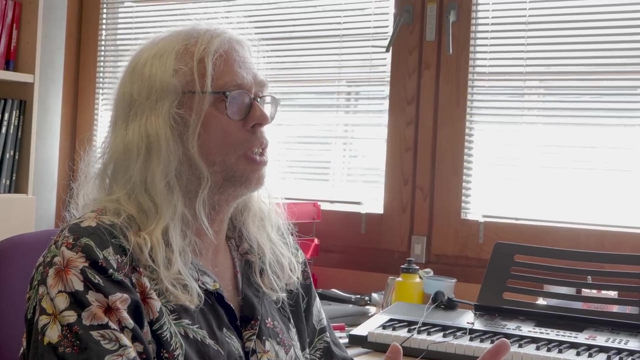 And goal's accomplished, I get a firework and I can get rid of my sorry because I have done the whole proof. So that's an example of a very simple proof. This is one of these warm-up exercises to prove these propositional tautologies. 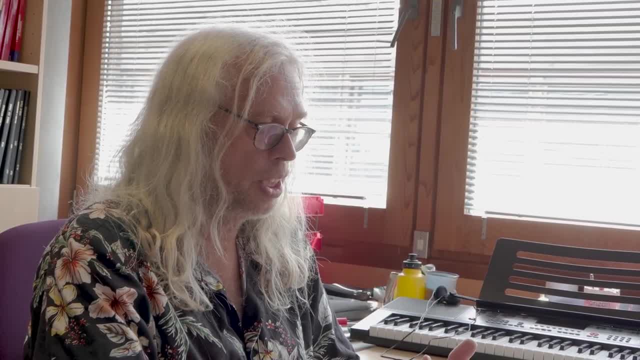 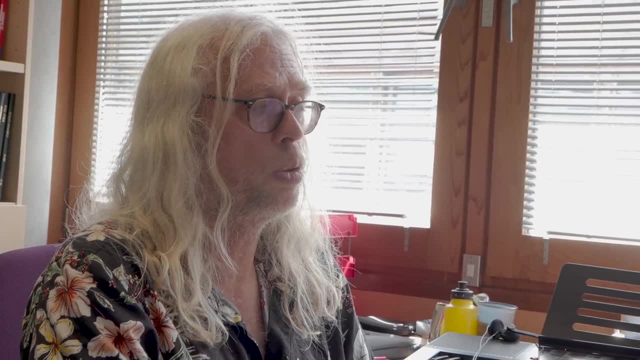 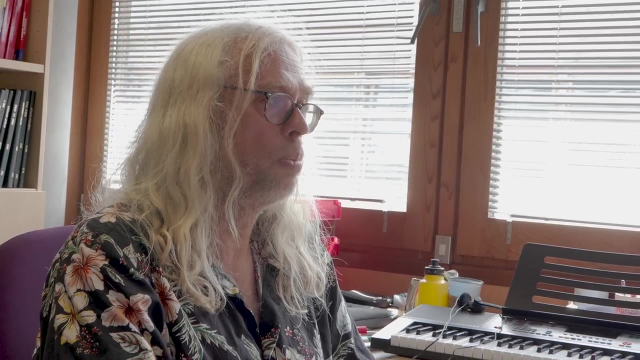 which are, as I say, it's a pattern of reasoning, right? We learn things like: okay, if you want to prove not, Q implies not P, then you can prove P implies Q. Okay, Now, this is a very simple. 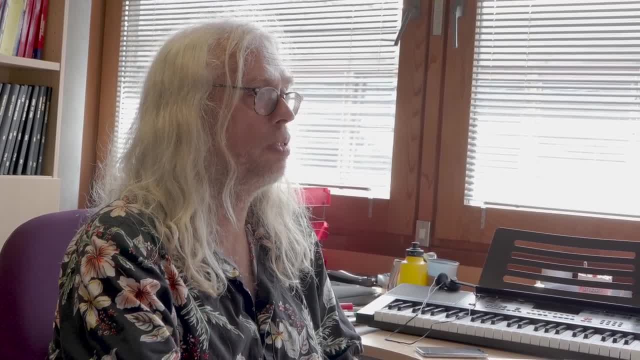 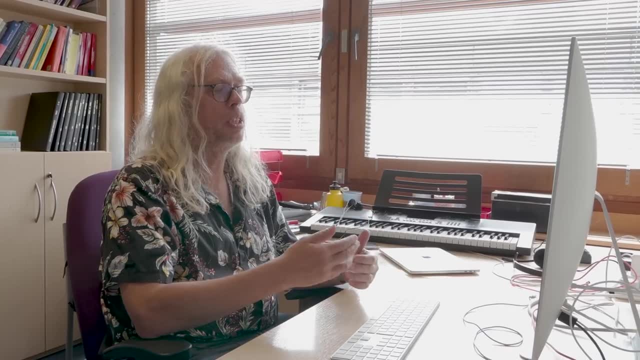 very simple tautology. And you think: why do I have to invest all this hard work to do this? And the answer is: you don't. So Lean has a built-in prover which can, which can automatically prove very simple propositions. 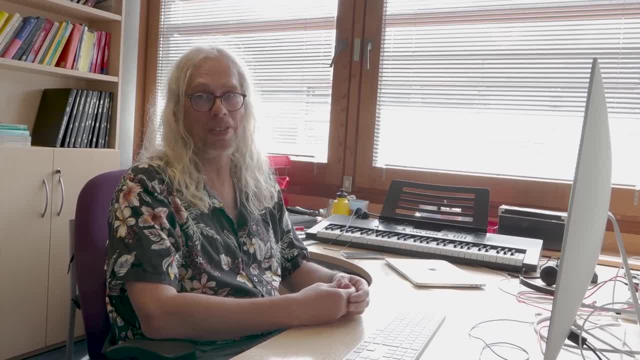 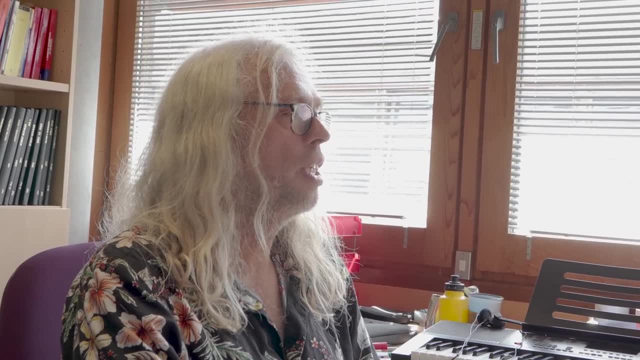 Now, if I want to teach people how to learn proofs, then they're not allowed to use IT. This is like having a pocket calculator. Yeah, yeah. yeah, It's like cheating, But I wanted to show something. Actually. what's a proof for Lean? 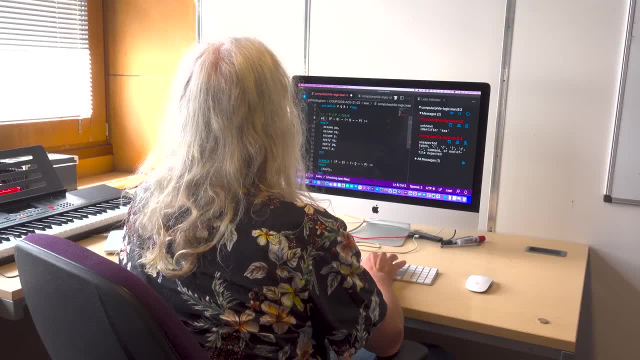 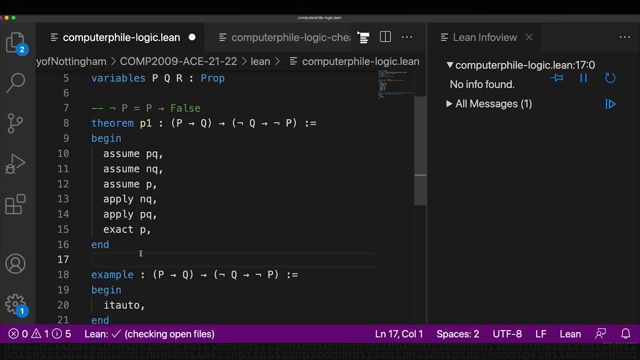 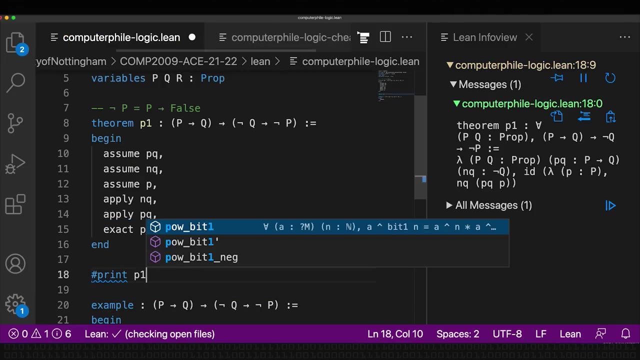 So here I just used example, but let me give this a name. Let's call it theorem P1.. Okay, So I've, we now prove the theorem and let's print the theorem. Okay, Or print the proofs actually, Okay, no comma. 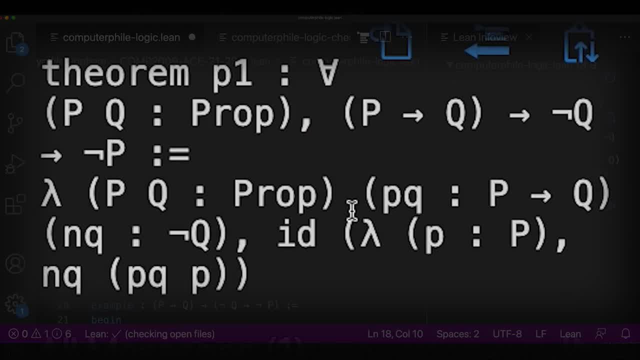 So here we see the proof in Lean, And then this is like a. it's actually a functional program. You see the lambda here. So it's a proof, It's a functional program, But I don't have to write this program.